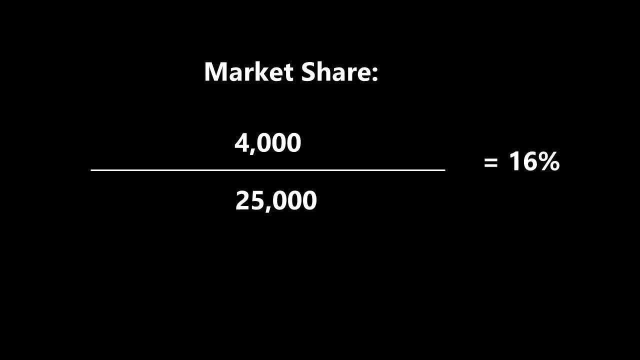 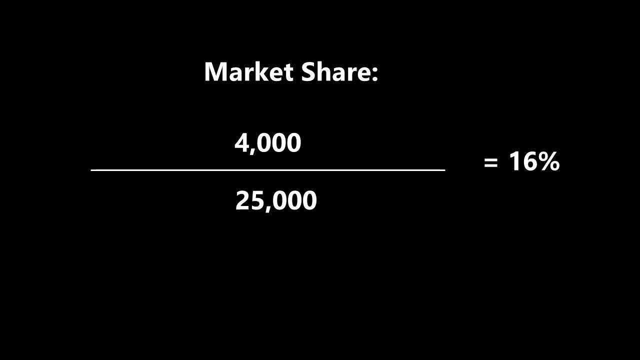 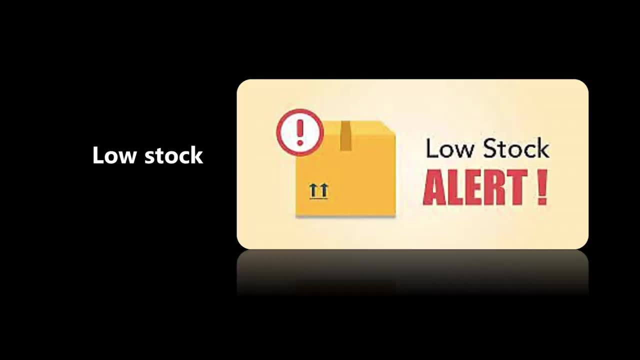 And usually there are four possible reasons for low market share. Like people don't know about our brand, that is, low brand awareness. low availability of stocks in the market. or people don't find that razors worthy of their money. That is, benefit deficiencies. or people could. 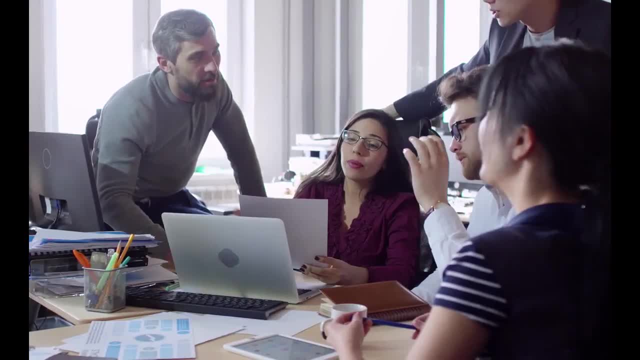 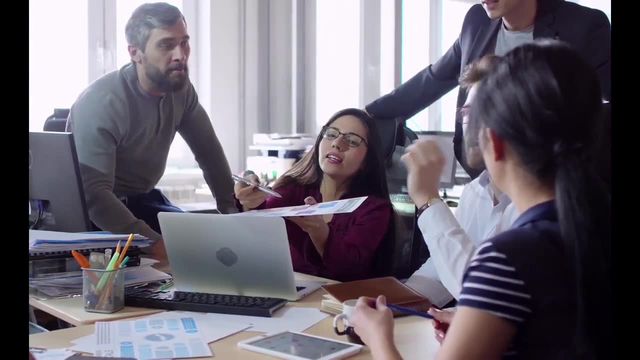 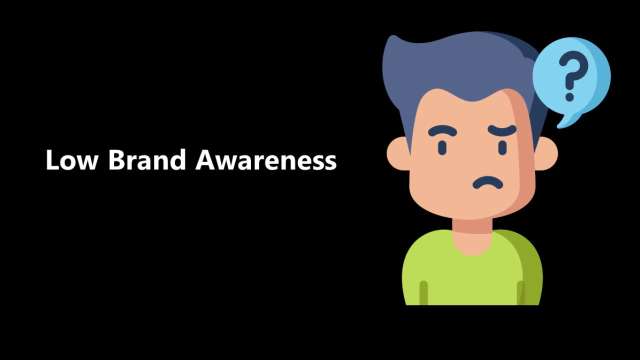 afford due to its high prices. to find out the exact cause of low sales, I had to address each possible reason and find out solving which one brings maximum increase in our sales. so after months of experimenting, we found out low brand awareness was the reason. that's when we wanted to do what anizer bush did, when 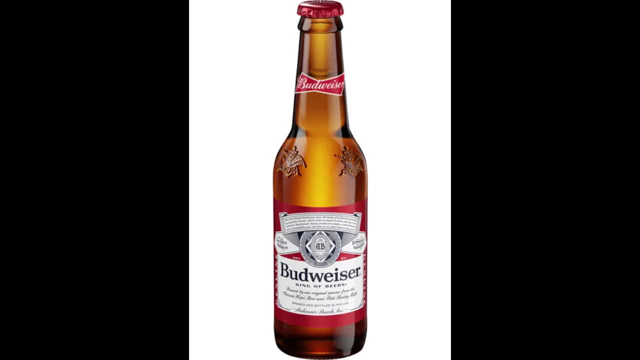 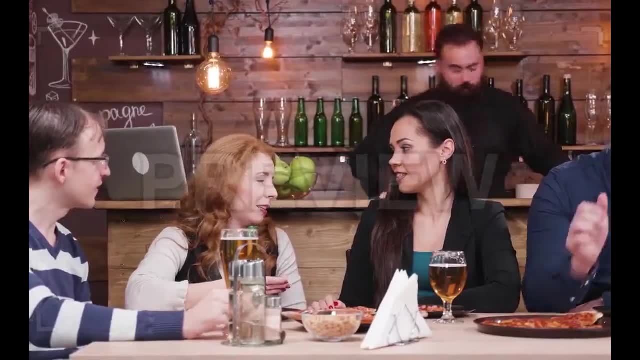 they face the same problem with one of their brands called Budweiser, the most popular beer brand in the world but apparently was not popular enough among the growing Hispanic population of Texas. it was a demographic market where Budweiser was underperforming and as a worsted number of special marketing. 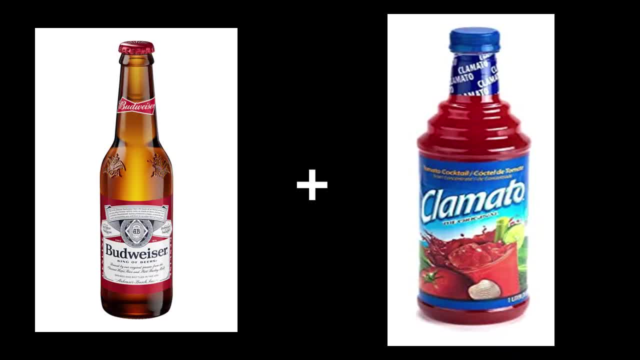 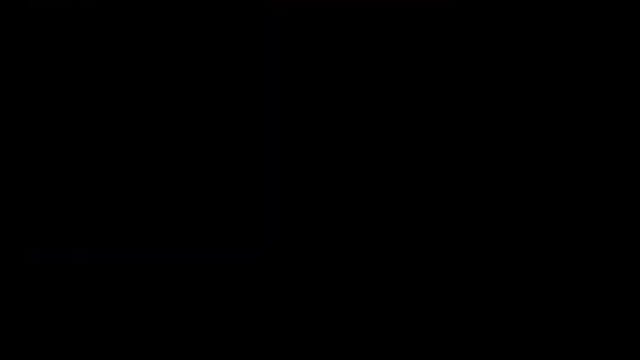 activities like cross promotion of Budweiser with Clamato tomato clan cocktail, a drink that is consumed in tens of millions of gallons every year in America, especially by Hispanics or Latin Americans. its sponsor, estinosa toca concert, which featured Latin Grammy Award singers and showed support to Latin heritage by supporting Latin music acts. all these 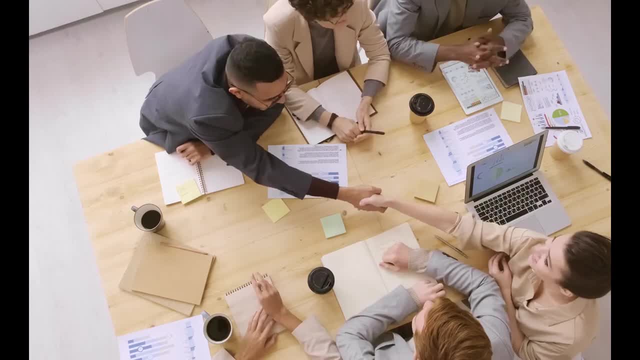 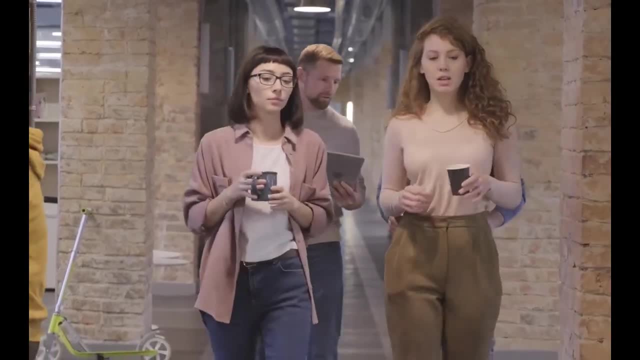 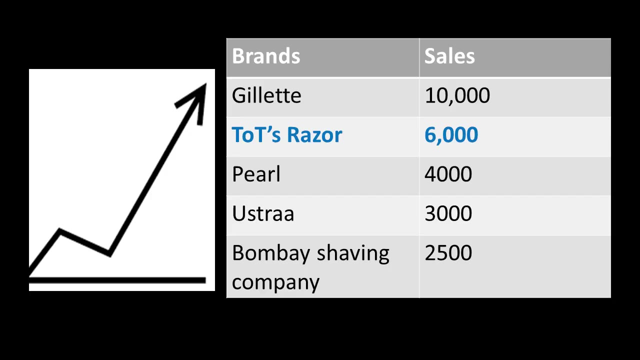 marketing activities contributed majorly to increase its sales by half a billion dollars in just one single year. so we decided to spend more on marketing by publishing ads on social media, local radios, local television channels of our city, the only place where we sell our razor blades. so you can see from the 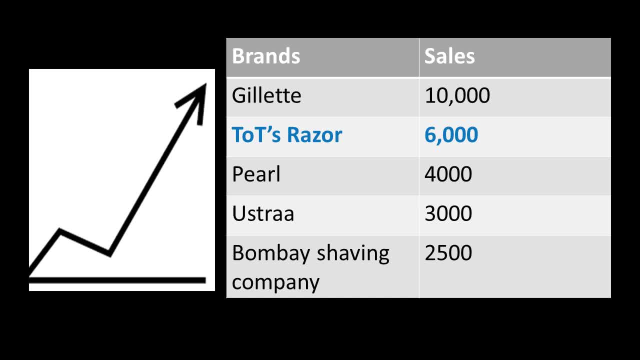 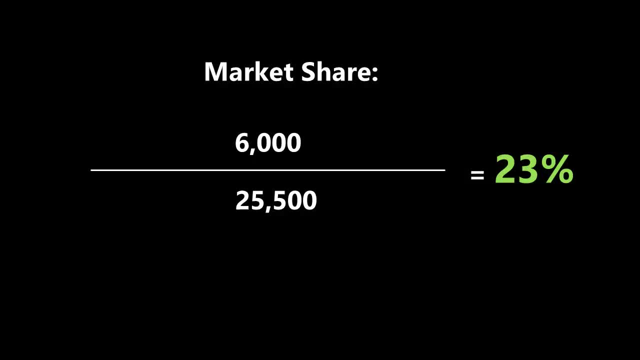 graph, our sales increased dramatically. we became the number two highest selling razor brand in our city, from number four. in a single year, this, out of fifty five thousand five hundred customers, we had twenty three percent of market share, up from sixteen percent in a year. we were able to do that because increasing brand awareness had a maximum impact on our 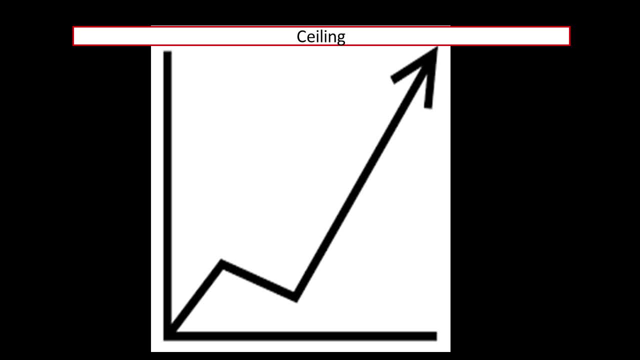 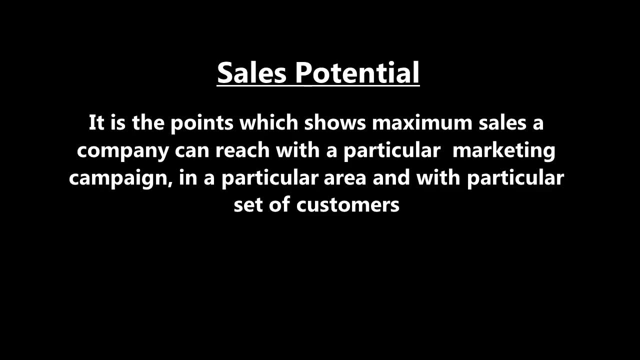 sales from out of all other reasons. but we soon reached a point. but no matter how many times you promoted of razors, the sales are not increasing, animal that is. we reach the point called sales potential. it has a point which shows maximum sales that company can reach with a particular marketing campaign. 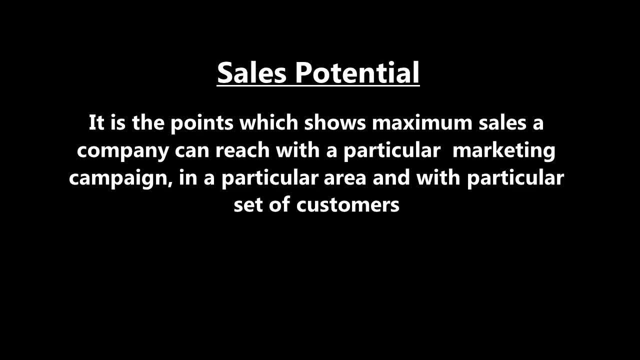 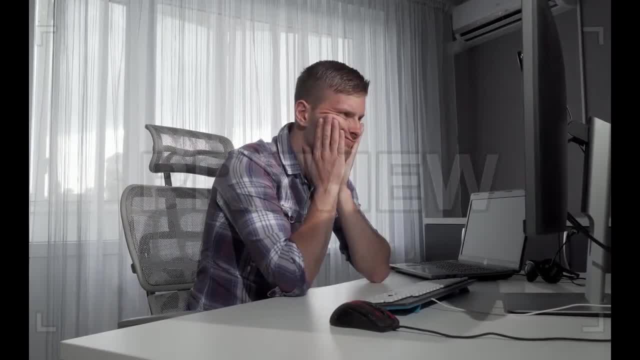 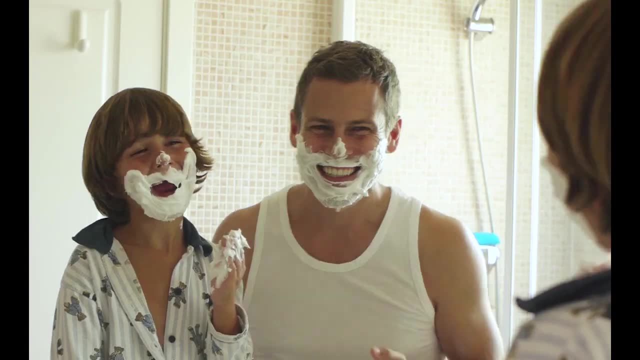 campaign in a particular area with particular set of customers. so that's it. it means, even after spending lakhs of rupees on marketing, 23 is the best that we could do. it's not about the razors when we started the company, but about the moments between a parent and a child where a parent looks. 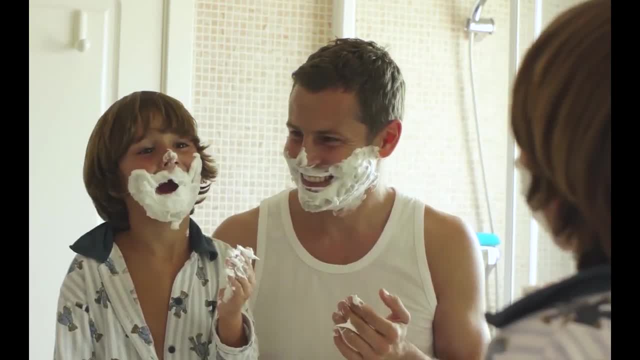 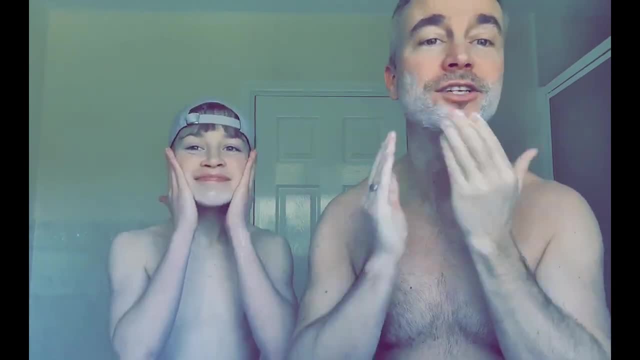 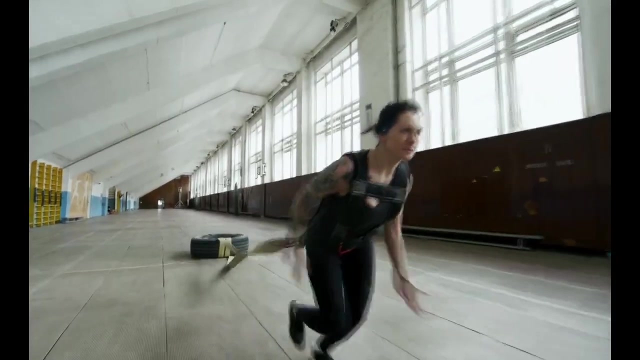 at his child, not as a kid but as an adult, and he wanted our products to be there in those moments and that teaching is kept. to shave with our razors was just a start, and our 23 percent is where we have to settle. it can't be the end right, not without a fight at least. so we dig a. 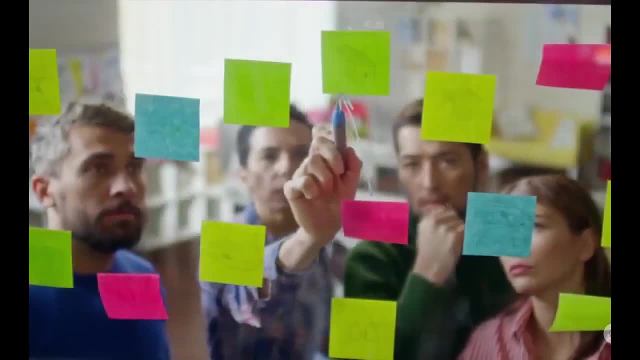 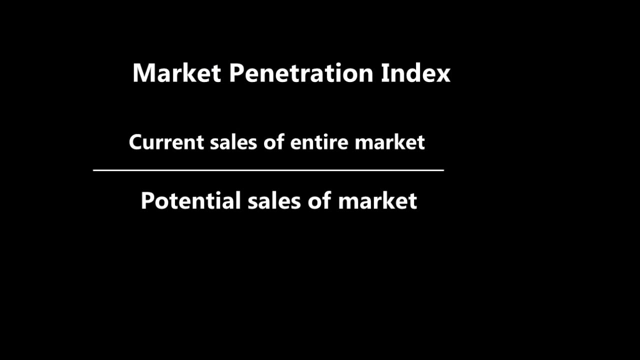 little deeper to find out what we could do to turn things around. so we calculated market penetration index. there's a ratio of current sales of entire market divided by potential sales of market. potential sales means sales revenue generated if every person- person who could use a razor- bought a razor instead of its substitutes like trimmers. 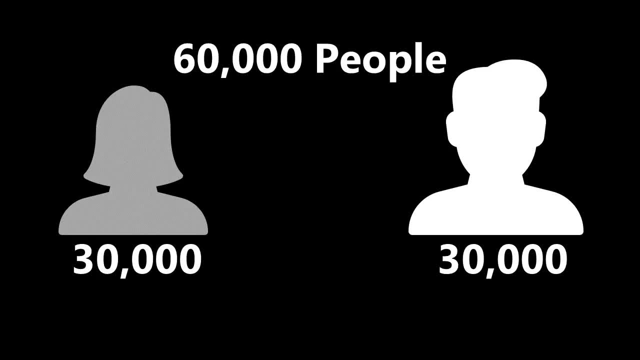 And that's when we found out the real problem. You see, there are 60,000 people living in a city. Half of them are women, so other half 30,000 men are our targeted demographic segment. But men who use razors are typically about 20 years of age on an average. 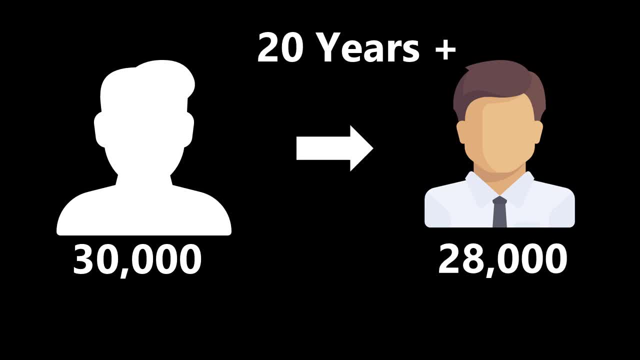 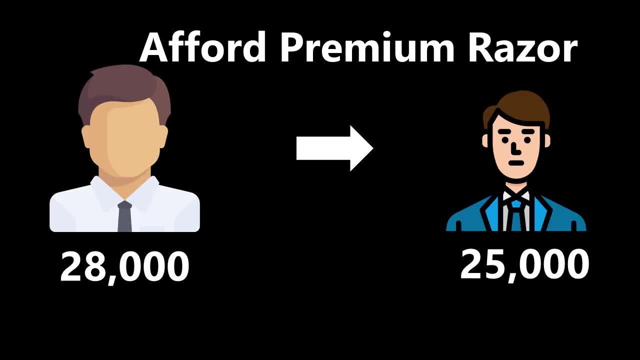 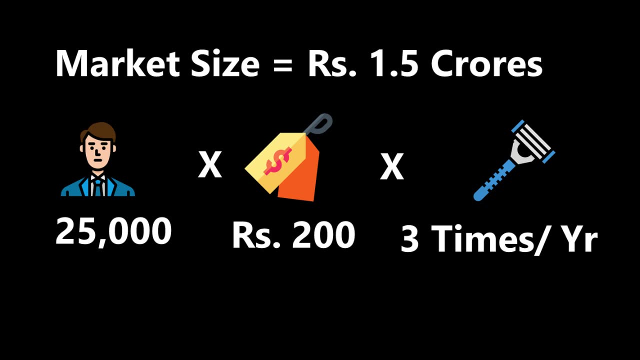 That brings our potential market to 28,000 from 30,000.. But since our brand, TOT's razors, are expensive, not all could afford it, So that brings our potential qualified customers to 25,000.. This brings the total market size to 25,000 customers. multiplied by 200 rupees, that is. 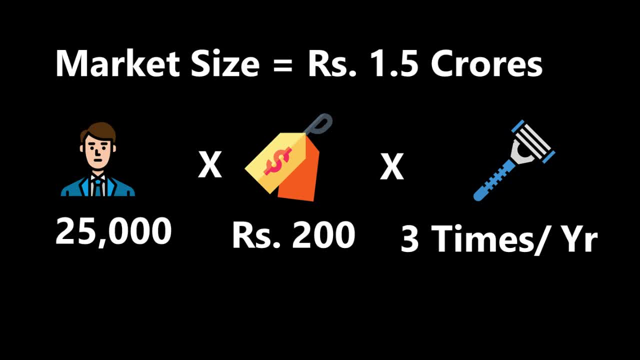 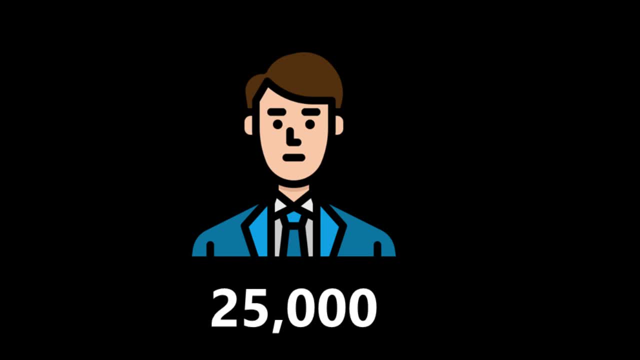 the price of razor blade into 3,. that is the number of times a new razor is purchased every year. This brings the total to 1.5 crores, Since all other factors are hard to change. so all the companies compete for these 25,000. 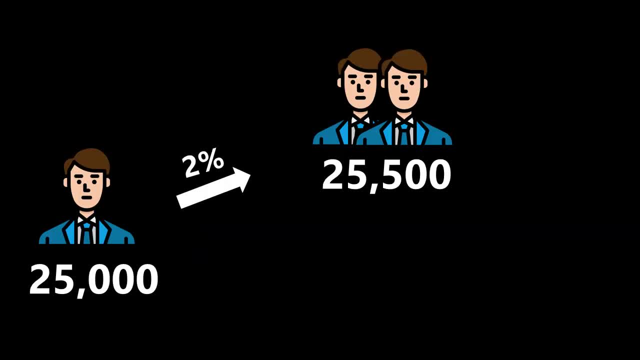 customers. But the problem is only 2% new customers. That is only 2%. kids start using razors every year. Now, if the market is not growing fast enough, how could we expect to increase our sales at a faster rate? There is no room for growth. 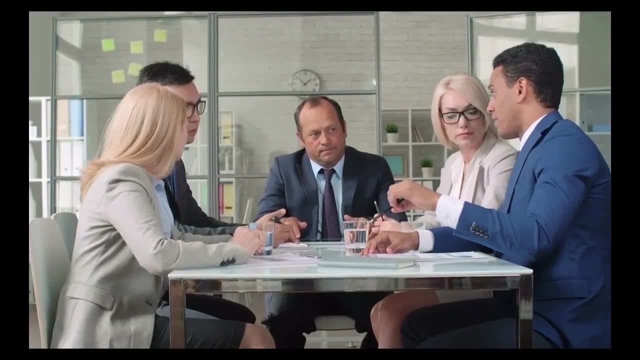 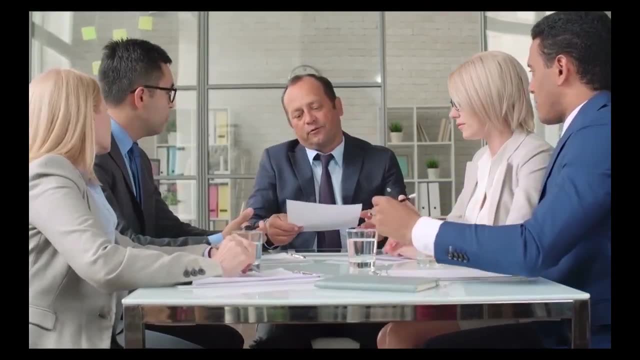 To know how bad the situation is. we calculated share penetration index Because we wanted to find out how much increase in our sales can we expect if we continue to use the same strategy? Share penetration index is the current sales of a company divided by potential sales. 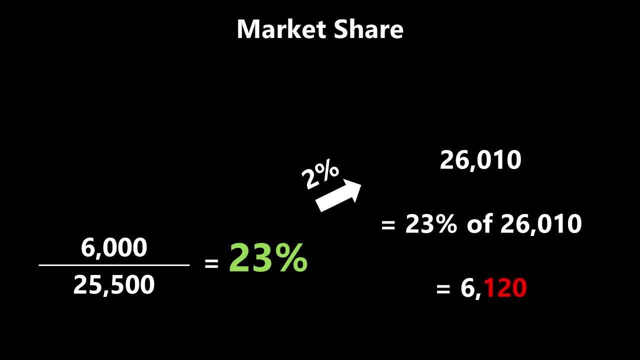 Our current market share is 23% And our potential market next year would be 26,010. that is 2% more than 25,500.. So 23% of 26,010 is 6,120. that is, only 120 more razors would be sold. 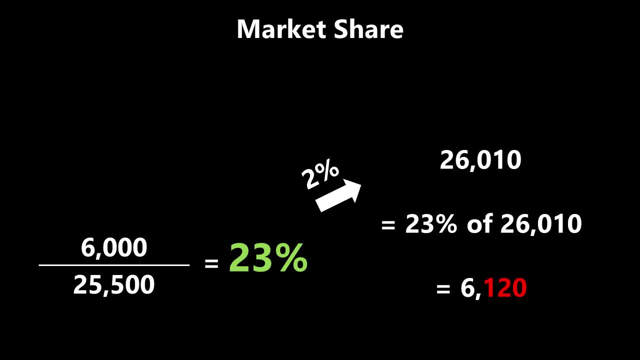 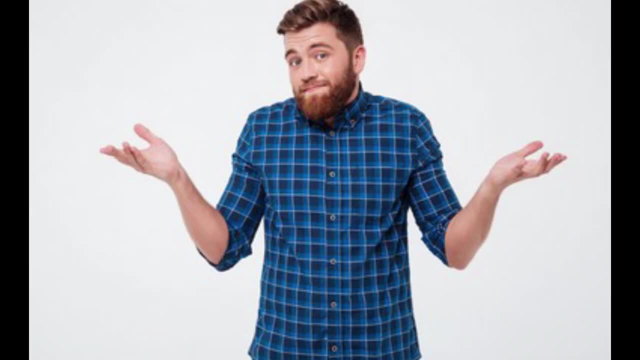 At this speed we would go bankrupt. So we have to do something, and fast. That's when it struck me: What if we increase our market itself? Market demand is made up of 4 elements: 1. People who want our product and could afford it. 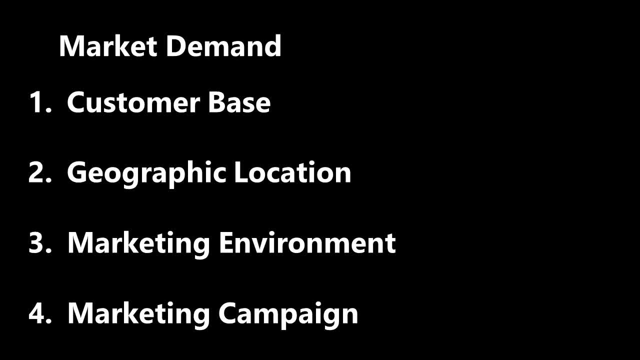 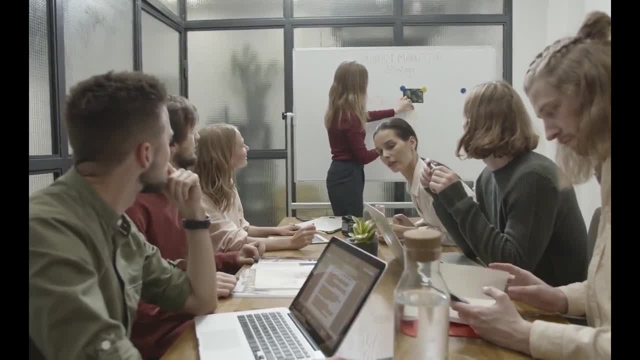 2. Geographical location. 3. Marketing environment and marketing campaign. We changed our marketing campaign by publishing ads on social media, local TV channels and radio, But that couldn't increase our market share about 23%. We can't change marketing environment, that is, economic conditions of people, political. 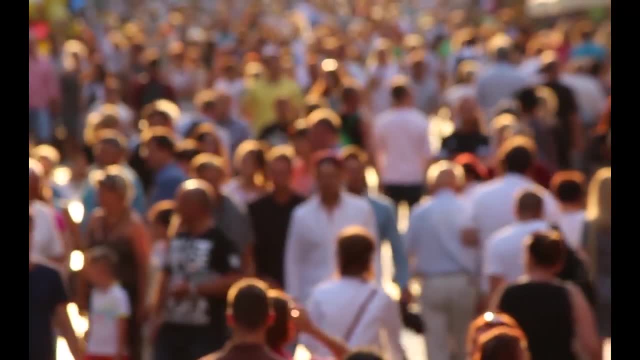 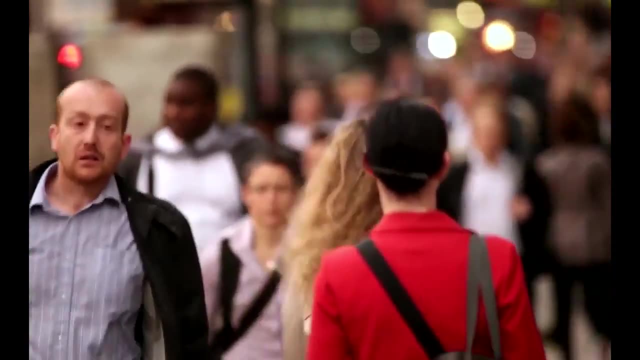 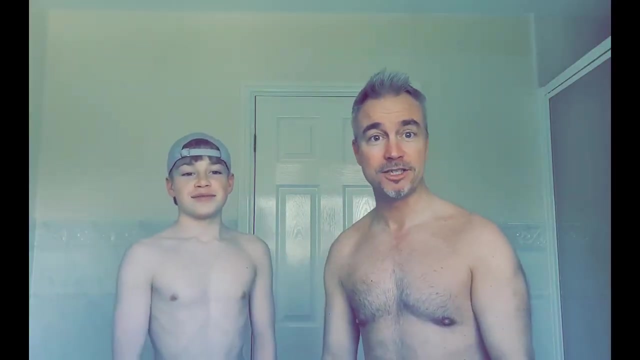 environment or technological environment. We cannot lower our prices for more men to afford it because we couldn't cover our cost. We could sell in neighboring cities. But there's other aspect That will bring maximum impact: We could change our customer segment. We were primarily focused on men, because they are the head of the family and they are the 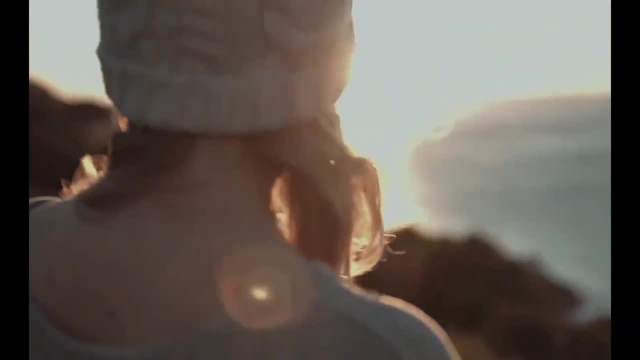 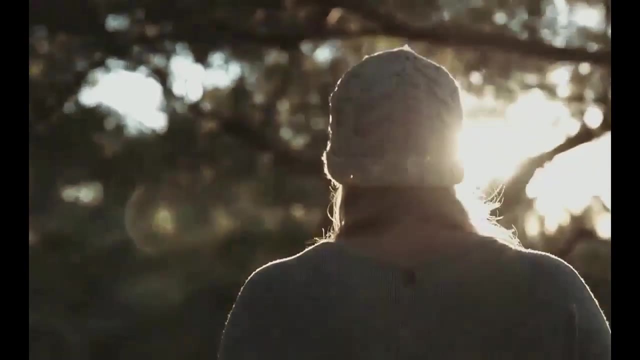 ones who use razors. But there is also a growing number of women who are now using razors instead of wax. So if we could tweak the razors to fit the requirement of women, we could add other half of the population of city, ie 30,000 additional potential customers. 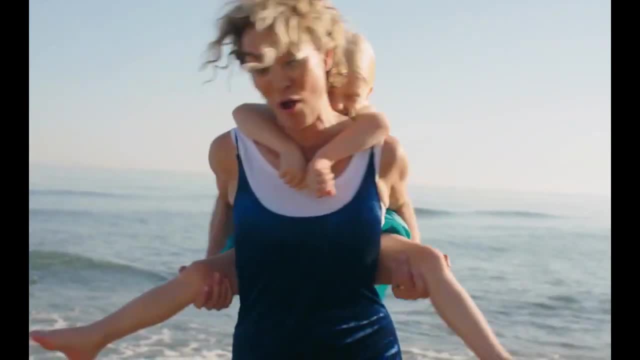 After all, men are not the only one who are responsible to protect their families. Men are not the only one who are responsible to protect their families. Men are not the only one who are responsible to protect their families. Women are the only one who are increasingly providing and protecting their families.